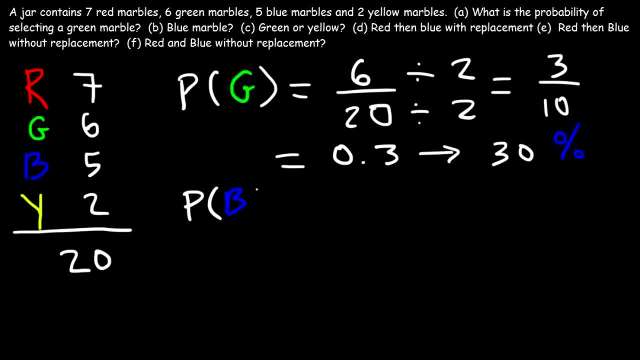 marble. So how many blue marbles are in the jar? Notice that we have five in the jar out of twenty. So the probability is five over twenty. So now let's reduce the fraction by dividing each number by five. Five divided by five is one. Twenty divided by five is: 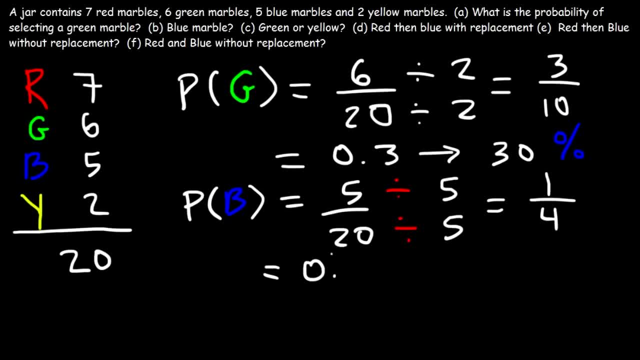 four, One over four, if you type it in the calculator, is .25 as a decimal, which correlates to twenty-five percent. So there's a twenty-five percent chance of selecting a blue marble. Now, if there's a twenty-five percent chance of selecting a blue, 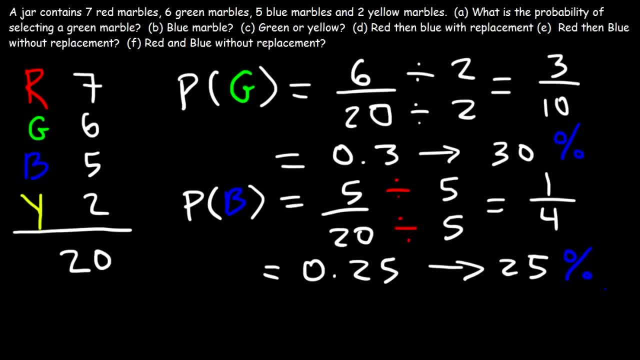 marble. what is the probability of not selecting a blue marble? To find the probability of not selecting a blue marble, it's going to be one minus the probability of selecting a blue marble, And the probability of selecting a blue marble is 0.25. 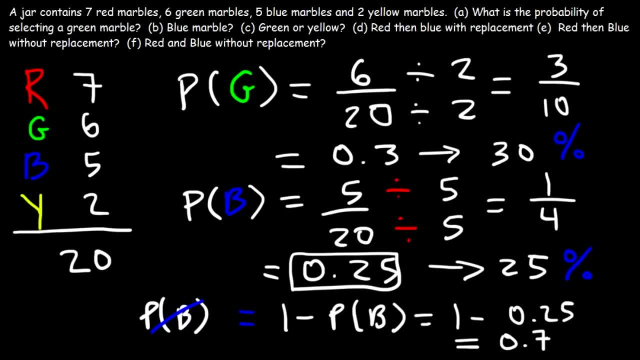 One minus 0.25 is equal to 0.75, which is 75%. So if there's a 25% chance of selecting a blue marble, then there's a 75% chance of not selecting a blue marble If there's a 30% chance of selecting a green marble. 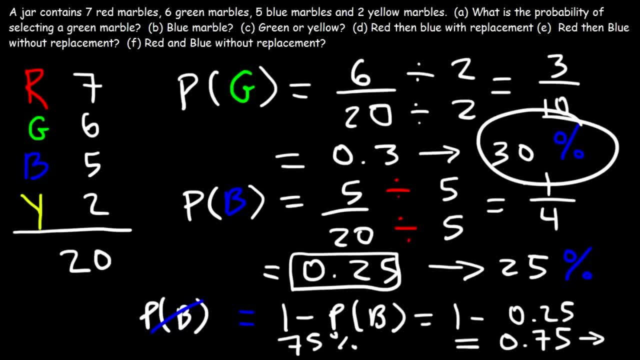 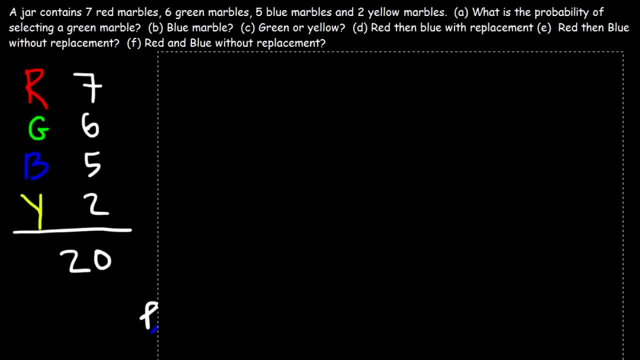 then there's a 70% chance of not selecting a green marble. Let's clear away a few things Now. let's talk about the probability of not selecting a blue marble. Let's talk about another way in which we can calculate the probability of not selecting a green marble. 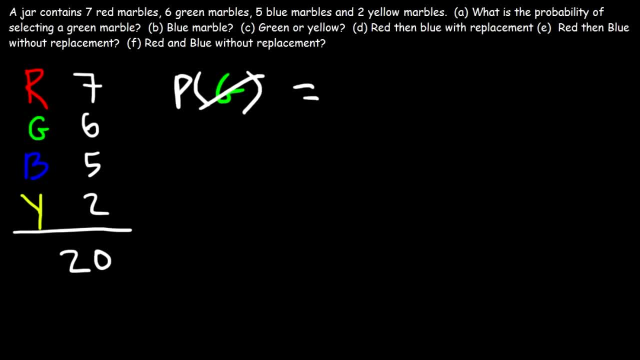 The other technique involves finding how many marbles are not green. So we have 7,, 5, and 2.. So that's 7 plus 5 is 12, 12 plus 2 is 14.. So there are 14 marbles that are not green. 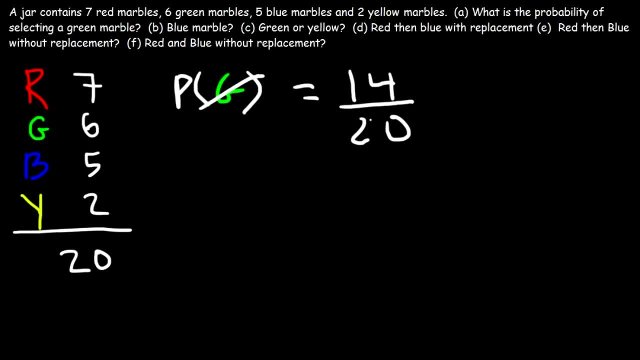 out of a total of 20.. And so let's go ahead and reduce this fraction. So let's divide both numbers by 2.. 14 divided by 2 is 7.. 20 divided by 2 is 10.. And so we get 7 out of 10,. 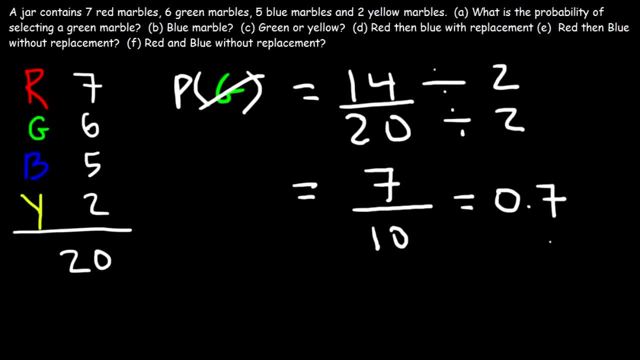 which is 0.7. And 0.7,. if you multiply by 100, you get 0.7. And 0.7,. if you multiply by 100, you get 0.7. And 0.7, if you multiply by 100,. 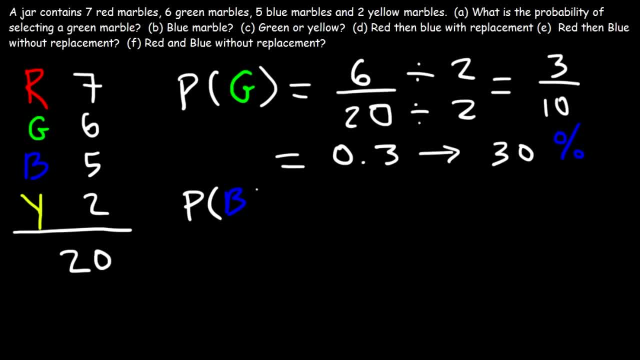 marble. So how many blue marbles are in the jar? Notice that we have five in the jar out of twenty. So the probability is five over twenty. So now let's reduce the fraction by dividing each number by five. Five divided by five is one. twenty divided by five is four- One over four, if you type. 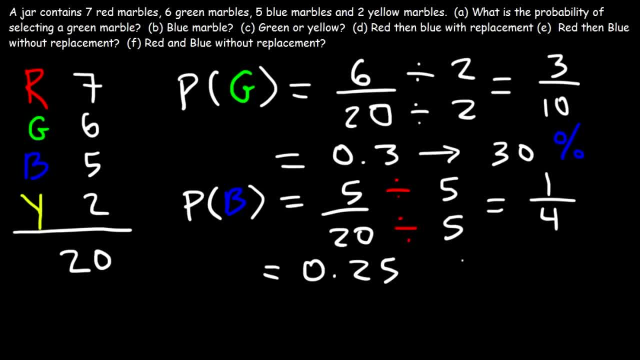 in the calculator is .25 as a decimal, which correlates to twenty-five percent. So there's a twenty-five percent chance of selecting a blue marble. Now, if there's a twenty-five percent chance of selecting a blue marble, what is the probability? 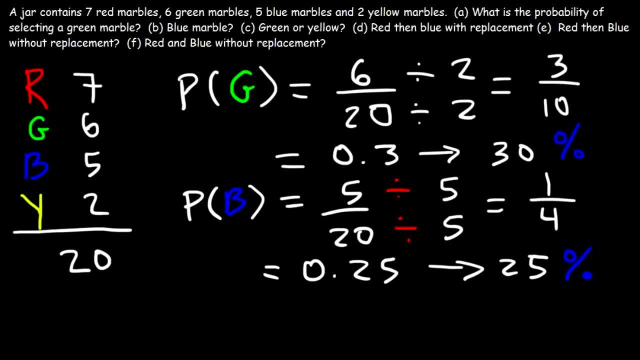 of not selecting a blue marble. To find the probability of not selecting a blue marble, it's going to be 1 minus the probability of selecting a blue marble and the probability of selecting a blue marble is 0.25, and 1 minus 0.25 is equal to 0.75, which is 75%. 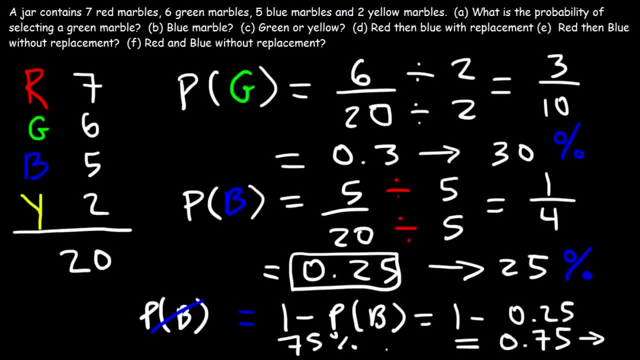 So if there's a 25% chance of selecting a blue marble, then there's a 75% chance of not selecting a blue marble. If there's a 30% chance of selecting a green marble, then there's a 70% chance of not selecting. 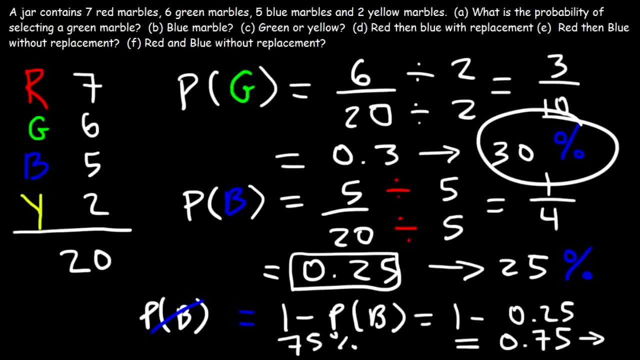 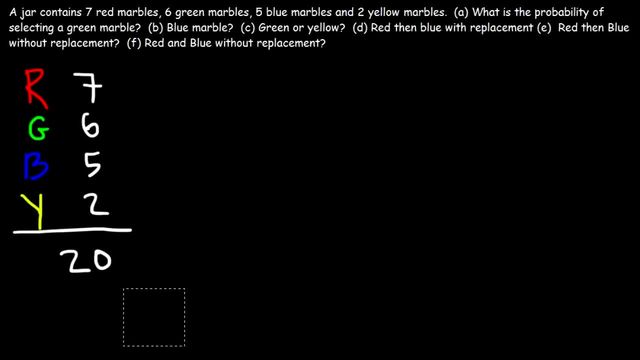 a green marble. Let's clear away a few things. Now. let's talk about another way in which we can calculate the probability of not selecting a green marble. The other technique involves finding how many marbles are not green. So we have 7,, 5, and 2.. 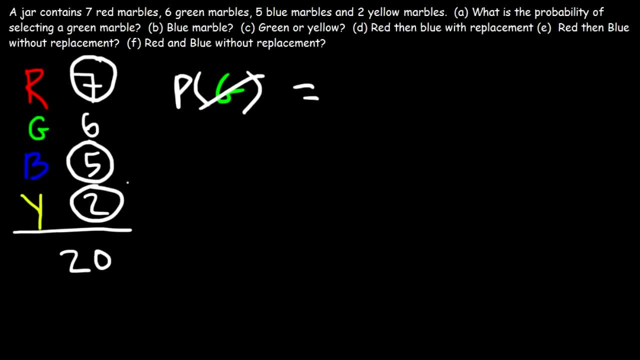 So that's 7 plus 5 is 12,, 12 plus 2 is 14.. So there are 14 marbles that are not green out of a total of 20.. And so let's go ahead and reduce this fraction. 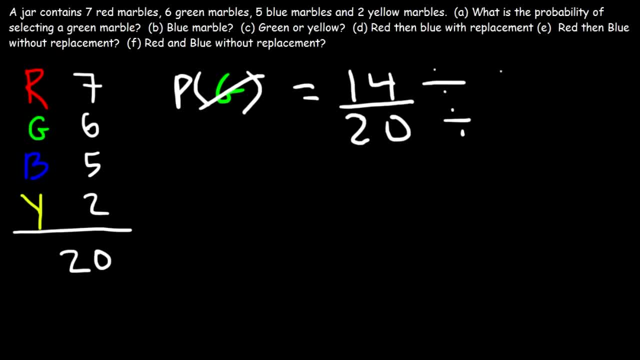 So let's divide both numbers by 2.. 14 divided by 2 is 7,. 20 divided by 2 is 10.. And so we get 7 out of 10.. And so we get 7 out of 10.. 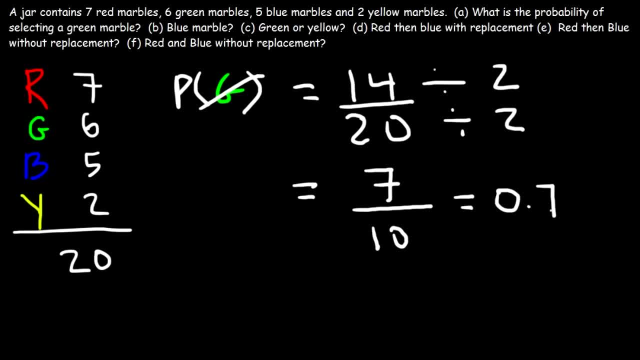 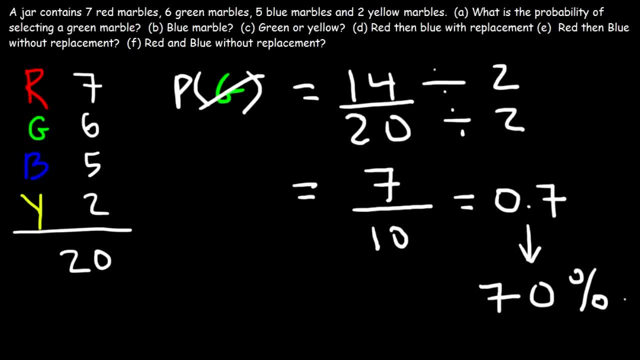 So, as you can see, there's a 70% chance of not selecting a green marble. Now, let's get rid of this. Now let's move on to the next part, part C: What is the probability of selecting a green marble? 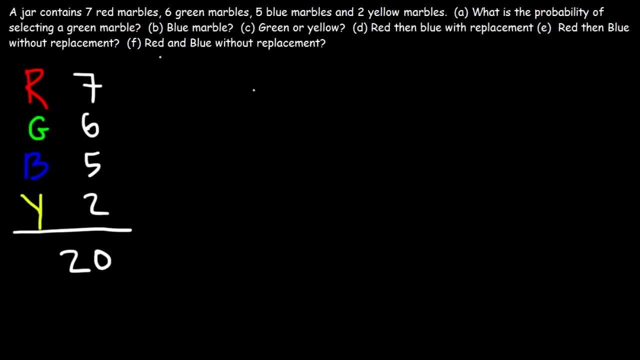 selecting a green or a yellow marble. How can we figure this out? If you see an or statement, it's associated with the sum. The probability of selecting a green or yellow marble is equal to the probability of selecting a green marble plus the probability of selecting a yellow marble. So we just got to add. 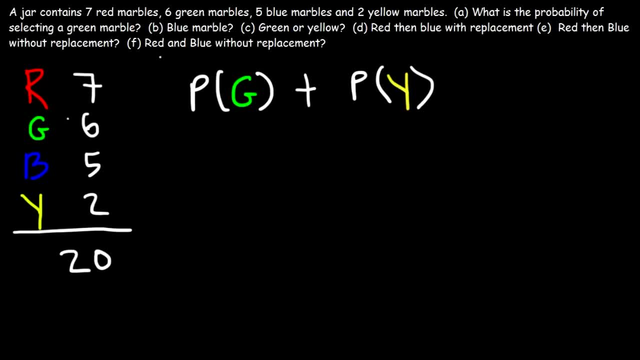 these two values and it's going to give us the answer. So there are six green marbles out of a total of 20 and to find a probability of selecting a yellow marble, we can see that there are two yellow marbles in the jar of 20 marbles. 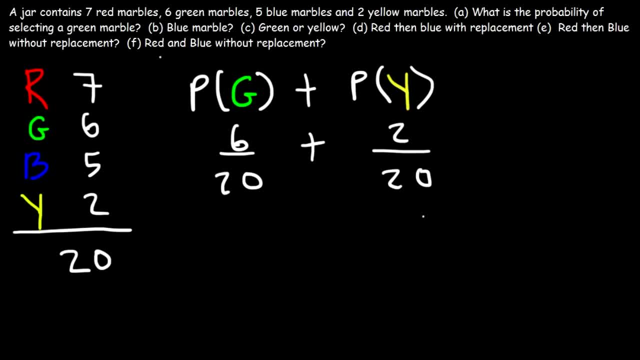 so it's two over twenty. now, Since the denominators are the same in these two fractions, we can go ahead and add them. Six plus two is eight, so it's eight over twenty. Now, eight into twenty years is equal to eight over twenty, So we just have to add. 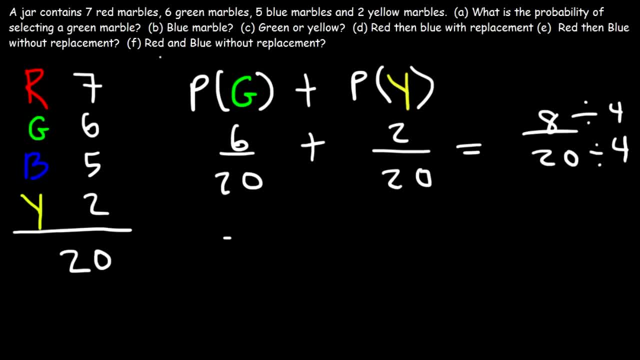 20 are divisible by 4, so let's reduce the fraction. so this is going to be 2 over 5. if you type 2 divided by 5 in your calculator, or if you use long division, you can convert this fraction into a decimal, and so it's going to be. 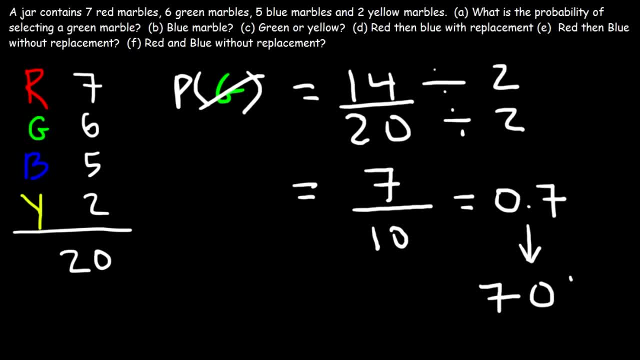 this will give you 70%. So, as you can see, there's a 70% chance of not selecting a green marble. Now, let's get rid of this. Now let's move on to the next part, part C. What is the probability of selecting a green or a yellow marble? 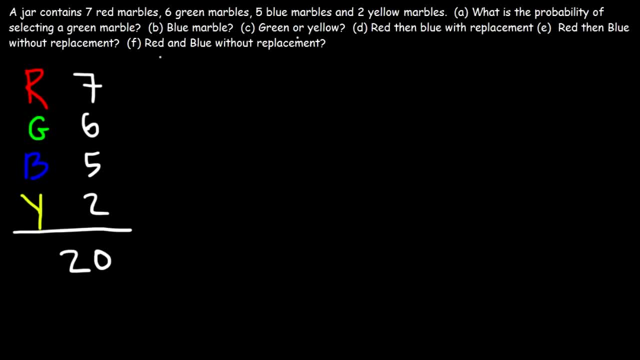 How can we figure this out? If you select a green marble, you see an or statement: It's associated with the sum. The probability of selecting a green or a yellow marble is equal to the probability of selecting a green marble plus the probability of selecting a yellow marble. 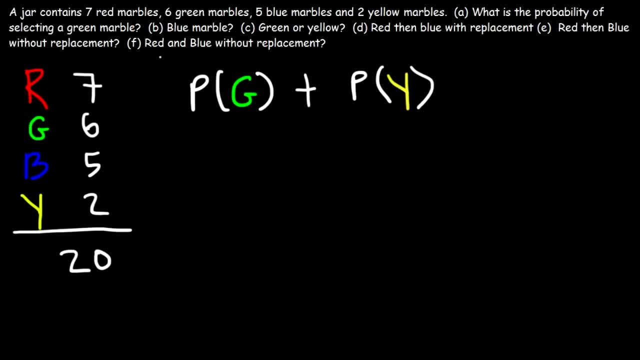 So we just got to add these two values and it's going to give us the answer. So there are six green marbles out of a total of 20.. And to find the probability of selecting a yellow marble, we can see that there are two yellow marbles. 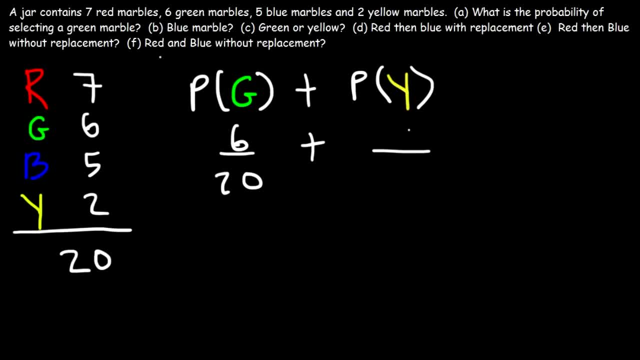 in the jar of 20 marbles. So it's 2 over 20.. Now, since the denominators are the same in these two fractions, we can go ahead and add them. 6 plus 2 is 8.. So it's 8 over 20.. 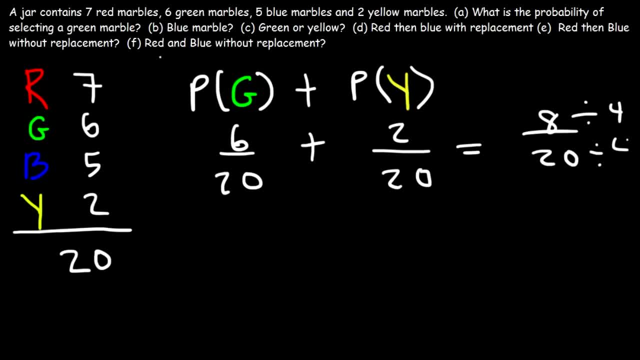 Now 8 and 20 are divisible by 4.. So let's reduce the fraction. So this is going to be 2 over 5.. If you type 2 over 5, 2 divided by 5 in your calculator, or if you use long division, 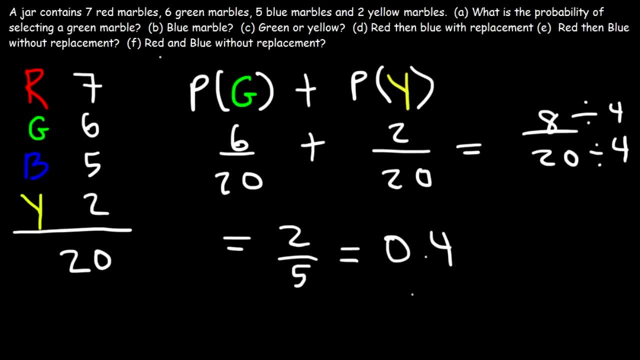 you can convert this fraction into a decimal, And so it's going to be 0.4, which is 40%. So there's a 40% chance of getting a green or a yellow marble. Now what about the next part? What is the probability of getting a red marble? 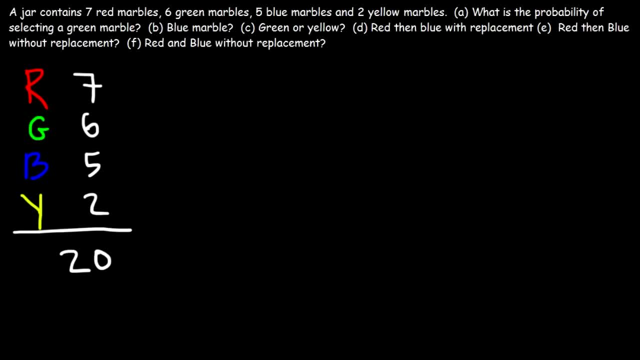 and then a blue marble with replacement. So this is basically an AND statement. We need to get red and blue. On the first try we need to get red, And on the second try we need to get blue. So the order matters here. 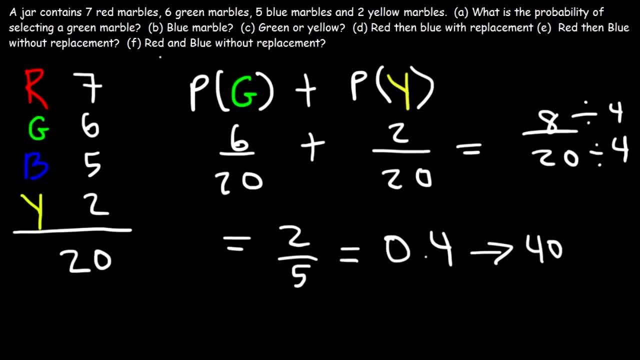 0.4, which is 40%. so there's a 40% chance of getting a green or a yellow marble. now what about the next part? what is the probability of getting a red marble and then a blue marble with replacement? so this is basically an and statement. we 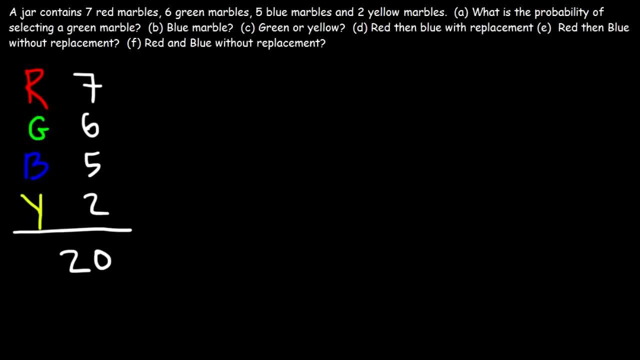 need to get red and blue. on the first try we need to get red, and on the second try we need to get blue. so the order matters here. so what is the probability of getting the blue marbled? we also need to get 3 towards the 3rd. now what you? 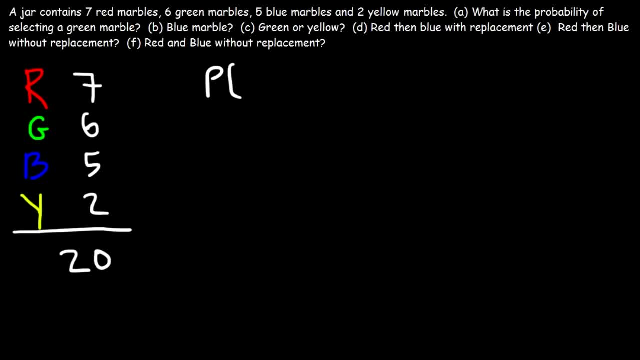 getting a red marble on the first try. by the way, whenever you have an and statement, you need to multiply. if there's an or you need to add, so just keep that in mind. so we need to multiply the probability of getting a red marble times the probability of getting a blue marble. so what is the probability of? 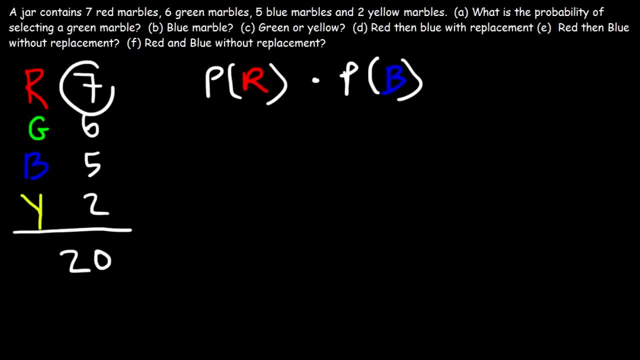 getting a red marble on the first try. so there's seven red marbles out of a total of twenty. so it's seven over twenty. now what is the probability of selecting a blue marble with replacement? with replacement means that once you take out the red marble in the first try, you put it back in and then you want to see you. 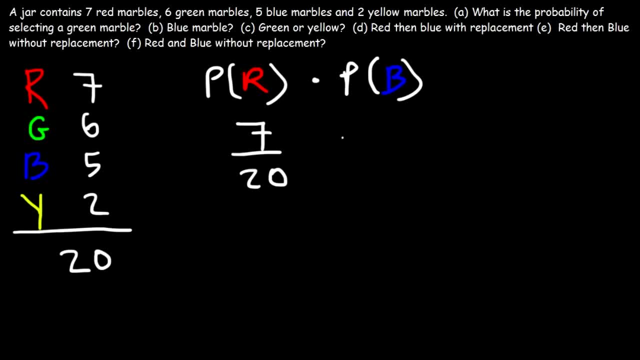 know the chances of getting a blue marble on the second try. so once you put the red marble back in, there's still a total of twenty blue marbles and there's five. I mean there's a total of 20 marbles in general and out of those 20 marbles we have five blue marbles. I think I said 20 blue marbles. 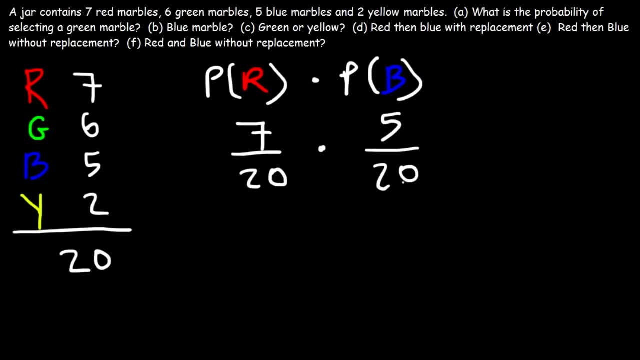 but there's only five. so once you put the red marble back in, you still have 20 marbles in the jar. now, instead of multiplying across, let's cancel first. we can reduce five over two, twenty. we can divide each number by five, so we can cancel off I from the top, and 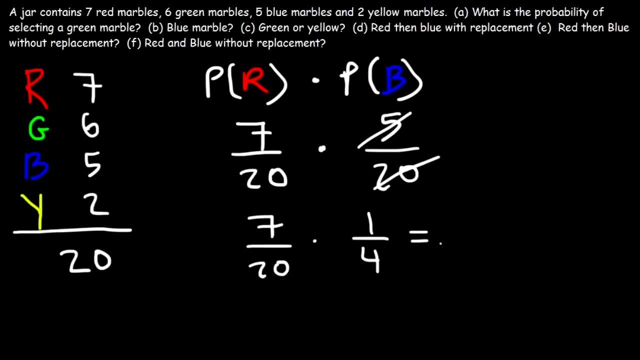 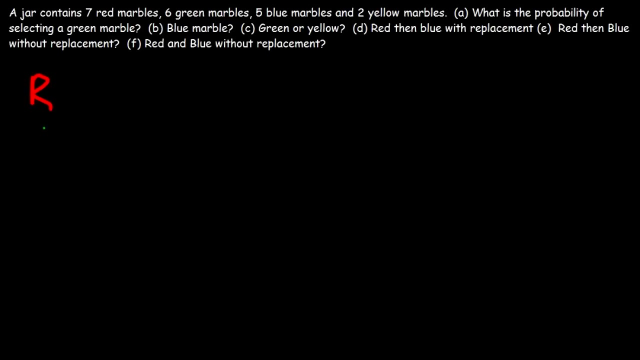 the bottom. so this is gonna be one over for seven times one is seven. seven times twenty is eighty. so the answer is seven over eighty and as a decimal this is equal to point zero, eight, seven, five, which is eight point seven five, tremendous percent. Now, if you're wondering what just happened, I accidentally closed the 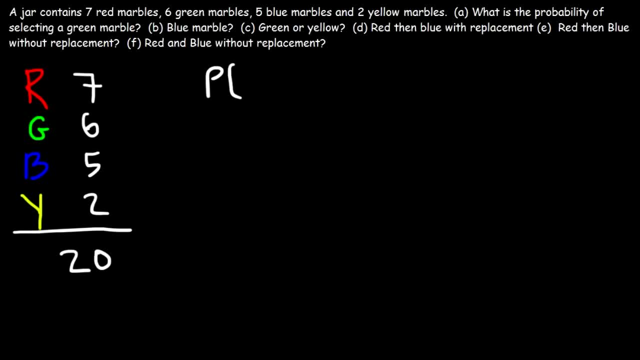 So what is the probability of getting a red marble on the first try? By the way, whenever you have an AND statement, you need to multiply. If there's an OR, you need to add. So just keep that in mind. So we need to multiply the probability. 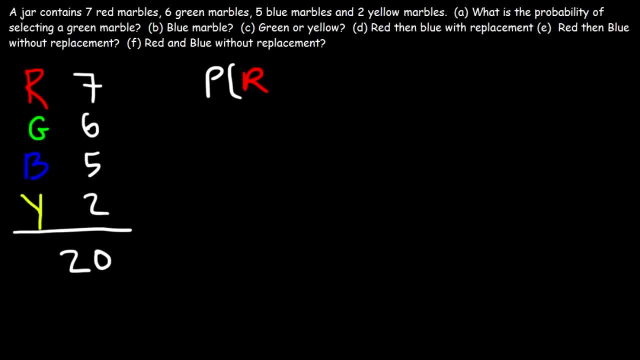 of getting a red marble times the probability of getting a blue marble. So what is the probability of getting a red marble on the first try? So there's 7 red marbles out of a total of 20.. So it's 7 over 20.. 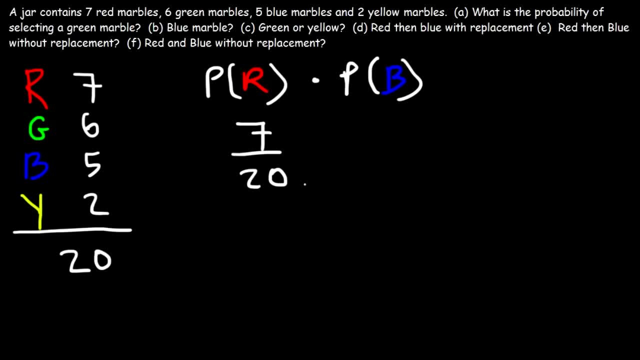 Now what is the probability of selecting a blue marble with replacement? With replacement means that once you take out the red marble in the first try, you put it back in And then you wanna see, you know the chances of getting a blue marble on the second try. 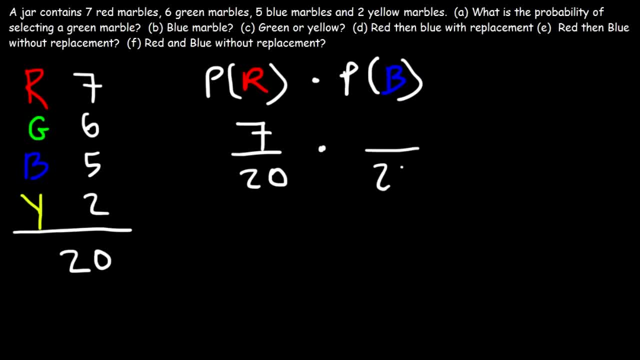 So once you put the red marble back in, there's still a total of 20 blue marbles And there's five. I mean there's a total of 20 marbles in general And out of those 20 marbles we have five blue marbles. 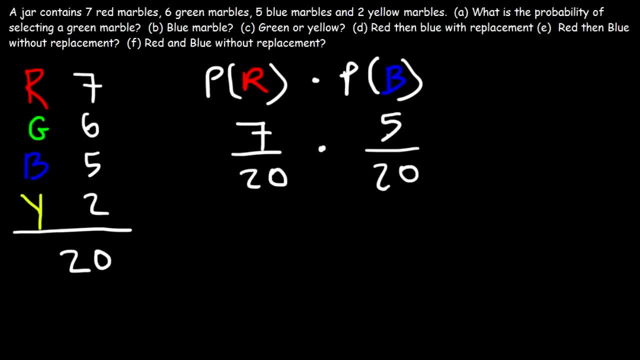 I think I said 20 blue marbles, but there's only 5.. So once you put the red marble back in, you still have 20 marbles in the jar. Now, instead of multiplying across, let's cancel first. We can reduce 5 over 20.. 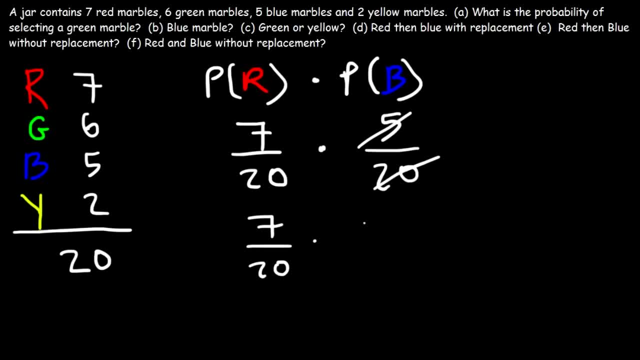 We can divide each number by 5.. So we can cancel a 5 from the top and the bottom. So this is gonna be 1 over 4.. 7 times 1 is 7.. 4 times 20 is 80.. 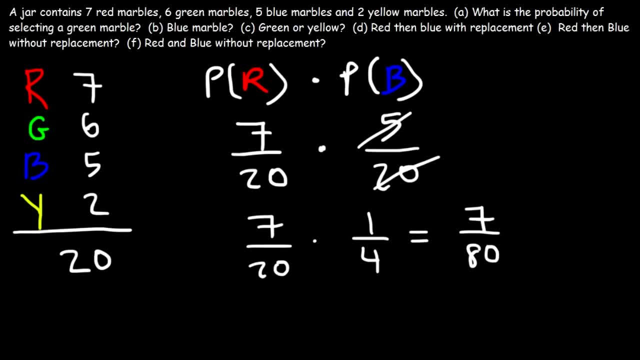 So the answer is 7 over 80. And as a decimal, this is equal to .0875,, which is 8.75%. Now, if you're wondering what just happened, I accidentally- I you know I got it wrong, but 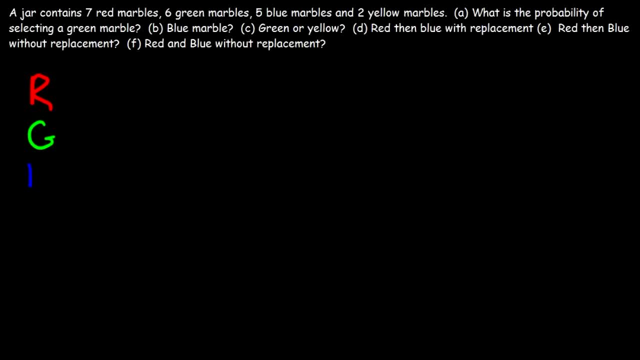 I accidentally. I got it wrong, but close the application, And so I'm just going to rewrite this information. But let's work on the next part. What is the probability of selecting a red marble and then a blue marble, but this time? 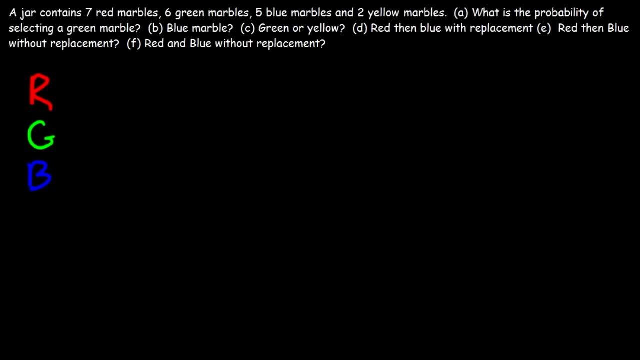 application, and so I'm just going to rewrite this information. But let's work on the next part. What is the probability of selecting a red marble and then a blue marble, but this time without replacement? So what do you think we have to do here? Feel free to pause the video and work on that example. So we're still. 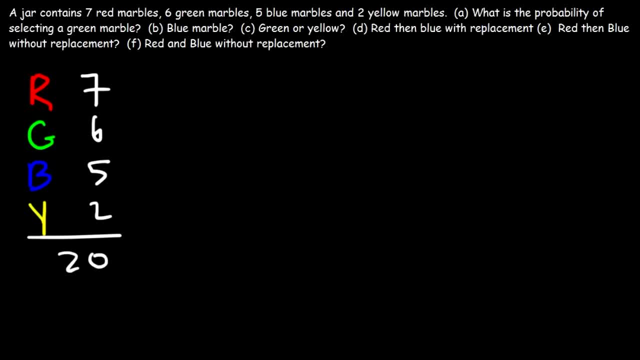 dealing with multiplication. There's two events. We need to get a red marble and a blue marble, And any time you're dealing with an AND statement in regards to probability, you need to multiply the two events together, That is, you need to. 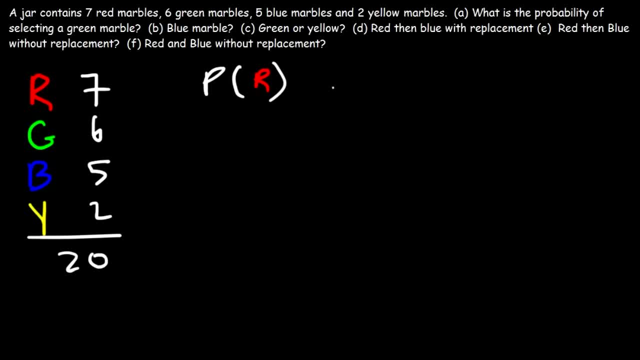 multiply the probability of getting those two events. so we need to get a red marble on the first try and then a blue marble on the second try. So the probability of getting a red marble on the first try is still 7 over 20, so that part hasn't changed. Now what about the probability of 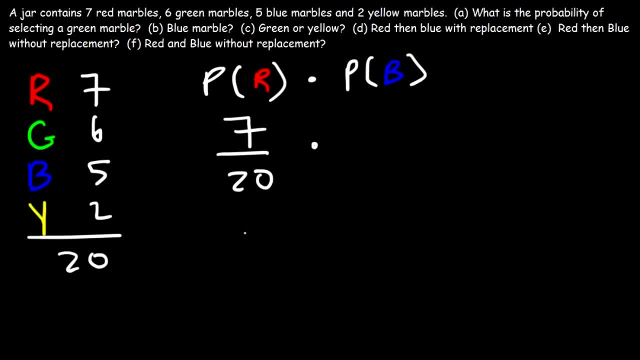 getting a blue marble, but without replacement. Without replacement means that after you take out the first red marble on the first try, you're going to get a blue marble on the second try. Now, what about the probability of getting a blue marble on the first try and then a blue marble on the second try? Well, if you 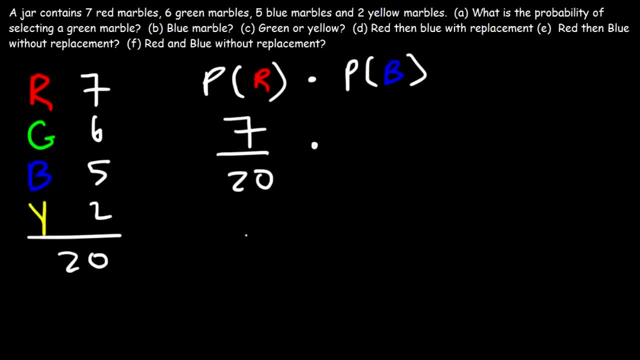 want to get it right on the first try. you don't put it back in, It stays outside of the jar, which means that we no longer have 20 marbles in the jar, we now have 19.. So therefore, the probability of selecting a blue marble is 5 out of 19,. 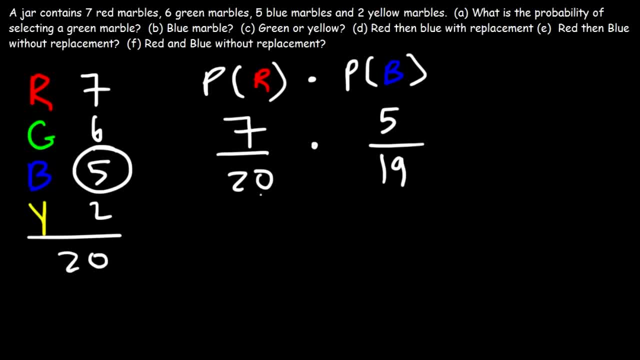 since there's five blue marbles in a jar that contains only 19 marbles left over, And so this is going to give us the answer. 20 is equal to the probability of getting the blue marble when the first try is done, not when the second try is last. 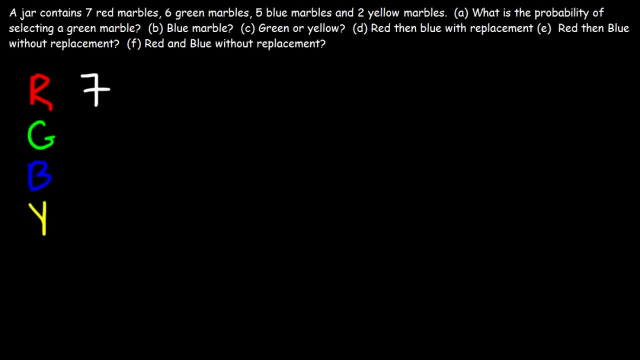 without replacement. So what do you think we have to do here? Feel free to pause the video and work on that example. So we're still dealing with multiplication. There's two events. We need to get a red marble and a blue marble, And any time you're dealing with an and statement in 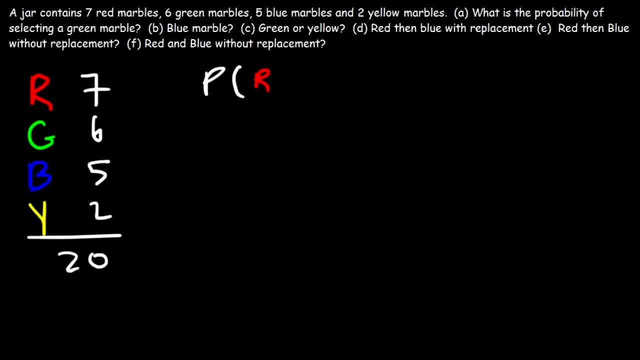 regards to probability, you need to multiply the two events together, That is, you need to multiply the probability of getting those two events. So we need to get a red marble on the first try and then a blue marble on the second try. 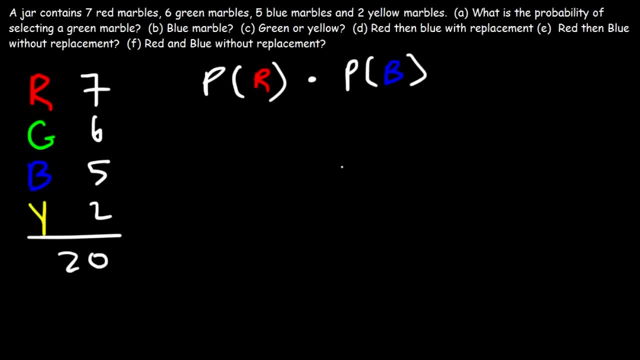 So the probability of getting a red marble on the first try is still 7 over 20.. So that part hasn't changed. Now what about the probability of getting a blue marble but without replacement? Without replacement means that after you take out the first red marble on the first try, 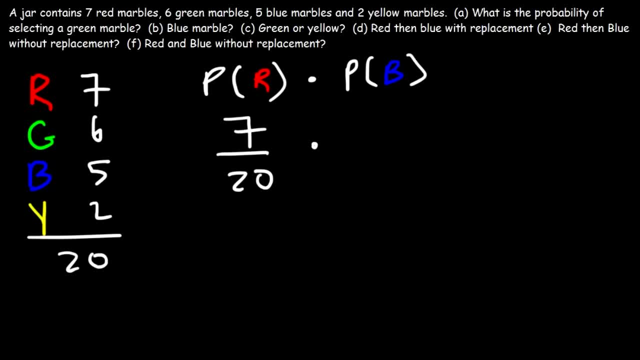 you don't put it back in, It stays outside of the jar, which means that we no longer have 20 red marbles. So we're still getting a red marble on the first try. So we need to multiply the probability of getting a red marble on the second try. We don't want to get a red marble on the first try. 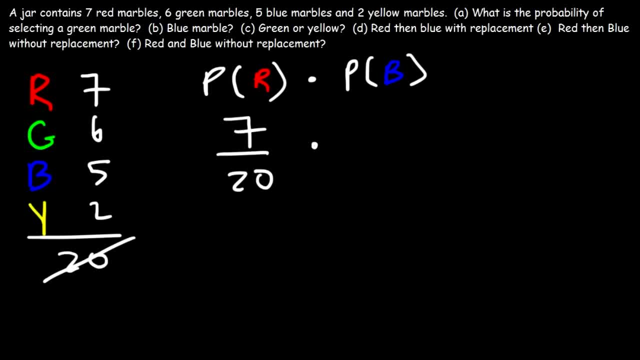 so that part is still the same. So we're still on the first try. There's still some demand for the blue marble, So now we have to multiply the probability of getting a blue marble. Now that we're out of the jar, if you take a blue marble, there are 5 out of 19.. The probability of getting a blue marble is 5 out of 19,. 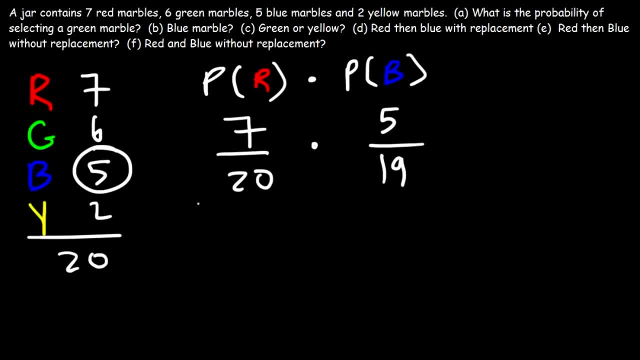 since there's 5 blue marbles in the jar, that contains only 19 marbles leftover, and so this is going to give us the answer. 20 is basically 5 times 4.. And notice that we can cancel a 5.. 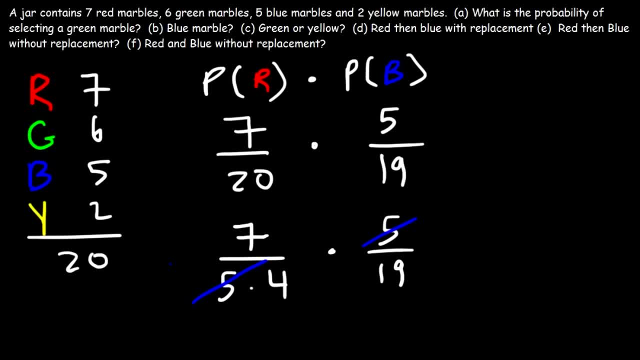 which will make the math a lot easier. so now on top is just going to be a 7 on the bottom 4 times 19. 4 times 19 is 76. 7 divided by 76 is point zero nine two. so there's a nine point two percent chance of getting a red marble on the first try. So how are we going to打 enduring a blue marble with these twoRAB has all these BLU MARBLES. Start this question and it will be pretty obvious sometimes that maybe it's a two-volume определization for any of those marbles. 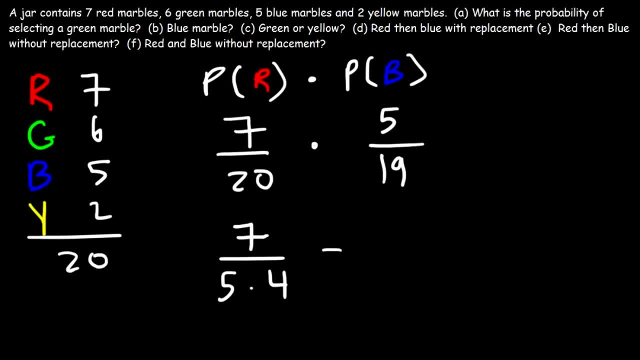 20 is basically 5 times 4.. And notice that we can cancel a 5,, which will make the math a lot easier. So now, on top, it's just going to be a 7.. On the bottom: 4 times 19.. 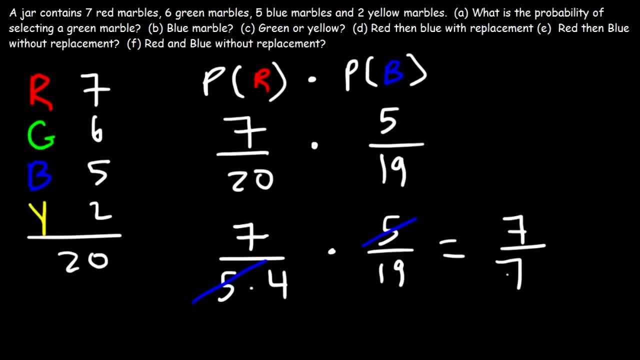 4 times 19 is 76.. 7 divided by 76 is 0.092.. So there's a 9.2% chance of getting a red marble on the first try and then a blue marble on the second try, without replacement. 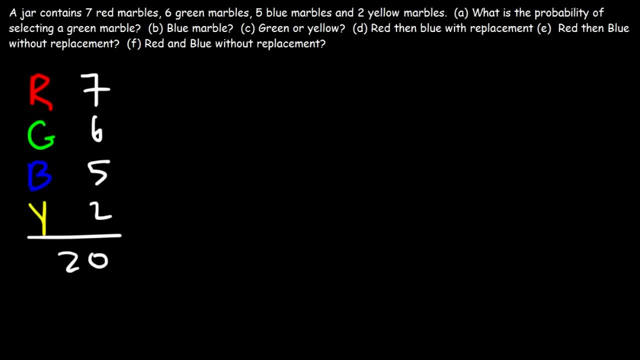 Now what about the last one? What is the probability of selecting a red marble and a blue marble without replacement? So how is part F different than part E? Go ahead, pause the video and think about this problem. See if you can get the answer. 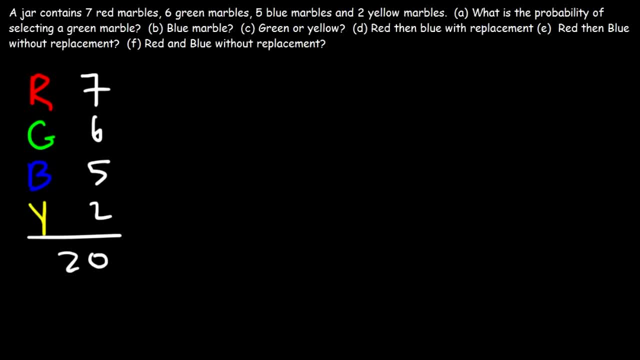 Try to work it out and then, when you're ready, unpause the video and see what the solution is. So what's the difference between then and and Now? in part E? on the first try, you want to get a red marble. 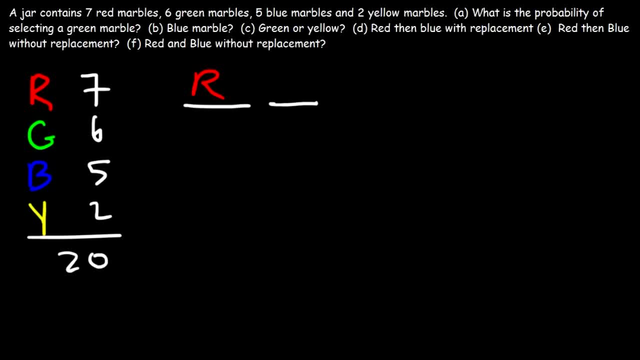 And on the second try you want to get a blue marble In that order. But in part F the order is not specified. So that means that you can get a red marble in the first try and then a blue marble in the second try. 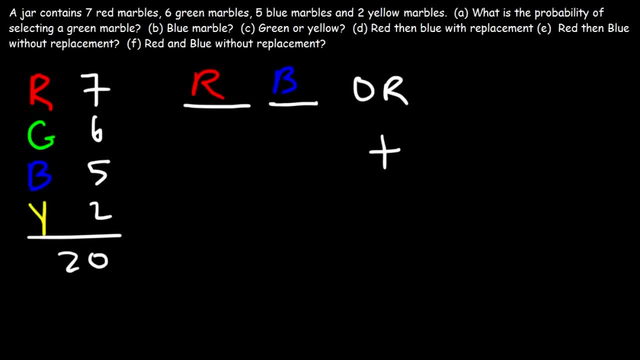 Or remember, or means plus or some. you can get a blue marble on the first try and then a red marble on the second try. In part F, because the order is not specified, it can be RB or BR. So the probability of getting red on the first try and then blue on the second try. 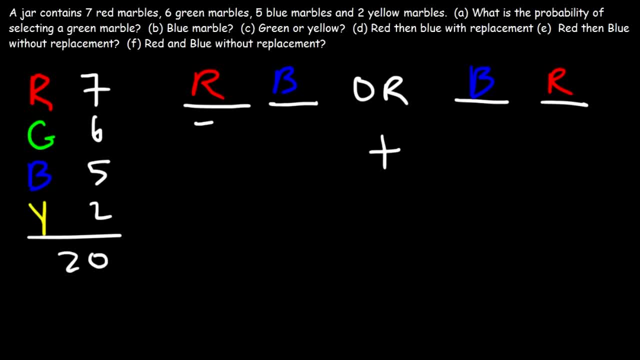 we got that answer in the last problem. It's 7 over 20 for the red marbles and then for the blue marbles it's 5 over 19.. This is without replacement, So don't forget to deduct this number by 1.. 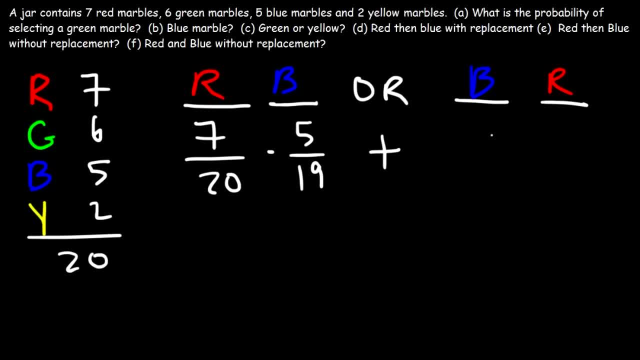 Now for BR, the probability of getting a blue marble. on the first try. there's 5 blue marbles out of a total of 20.. And since it's without replacement, once we take out the blue marble there's 19 left. 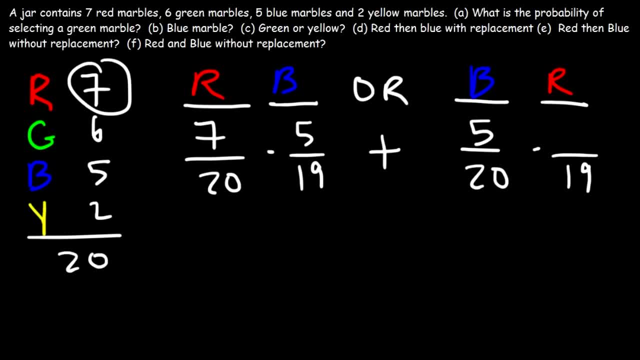 And the probability of selecting a red marble is going to be 7 out of the remaining 19.. So notice that these two answers are the same. In both cases we're going to get the same answer of 7 over 76. That's the probability of getting red, then blue. 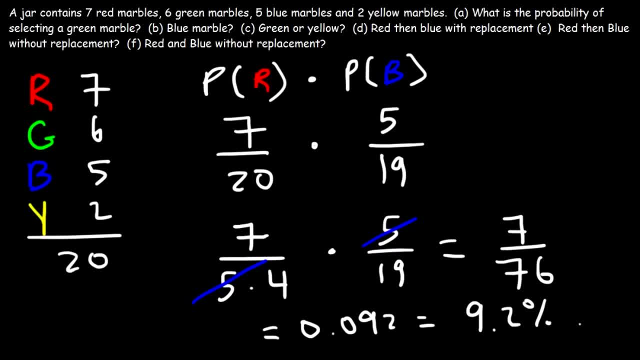 and then a blue marble on a second try, without replacement. now what about the last one? what is the probability of selecting a red marble and a blue marble without replacement? so how is part F different than party? you go ahead, pause the video and think about this problem. see if you can get the 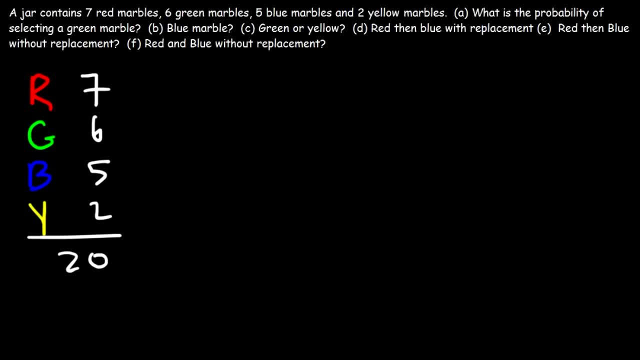 answer: try to work it out and then, when you're ready, unpause the video and see what the solution is. so what's the difference between then and and now in Part E? on the first try you want to get a red marble, and on the second try you. 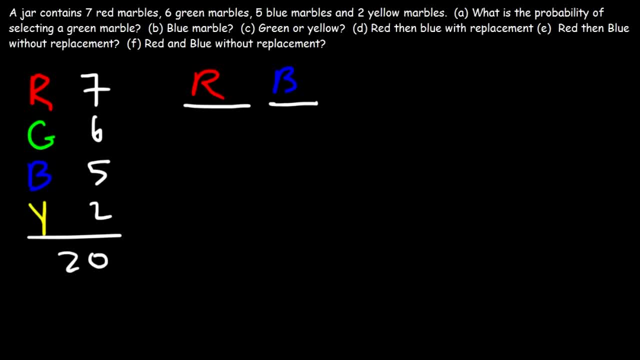 want to get a blue marble in that order, but in Part F the order is not specified. so that means that you can get a red marble in the first try and then a blue marble in the second try, or remember or means plus or some. you can get a blue marble on the first try and then a red. 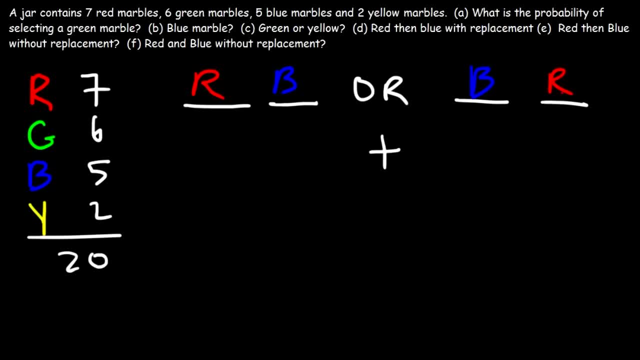 marble on the second try in Part F because the order is not specified. it can be RB or BR. so the probability of getting red on the first try and then blue on the second try- we got that answer in the last problem- it's seven over twenty for the red marbles and then for the blue Margo's it's 5 over 19. 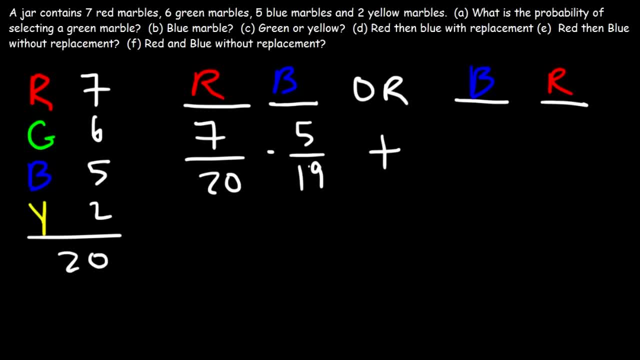 this is without replacement, so don't forget to deduct its number by one. now for BR, the probability of getting the blue marble on the first try. There's 5 blue marbles out of a total of 20, and since it's without replacement, once we take out the blue marble there's 19 left. 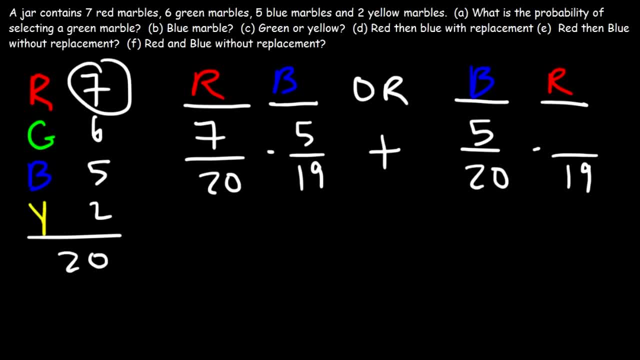 And the probability of selecting a red marble is going to be 7 out of the remaining 19.. So notice that these two answers are the same. In both cases, we're going to get the same answer of 7 over 76.. That's the probability of getting red then blue, and the probability of getting blue then red is also 7 out of 76. 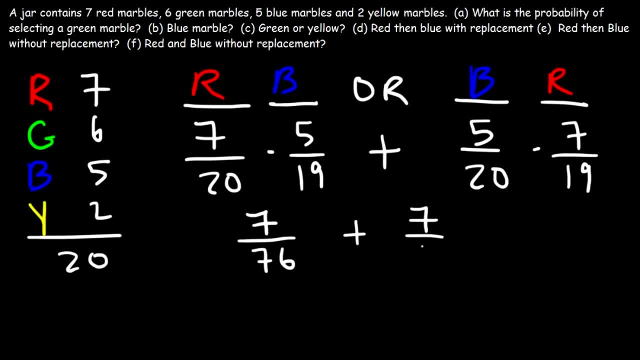 And the probability of getting blue then red is also 7 out of 76.. You have to double the answer, So it's 14 out of 76.. Now we can reduce this fraction. We can divide the top and the bottom by 2.. 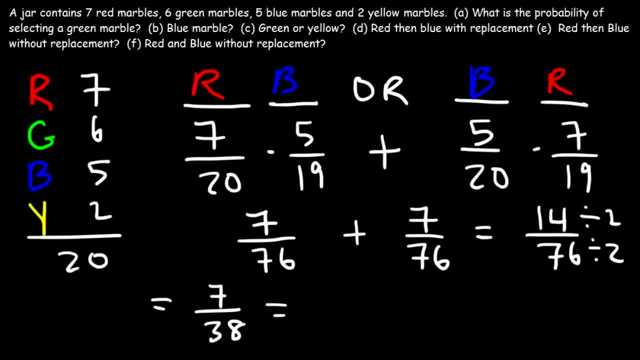 So this is going to turn into 7 over 38.. 7 over 38, that's 0.184 as a decimal, So there's an 18.4% chance of getting a red and a blue marble without replacement. The probability of not getting a red and a blue marble without replacement is 100 minus 18.4.. 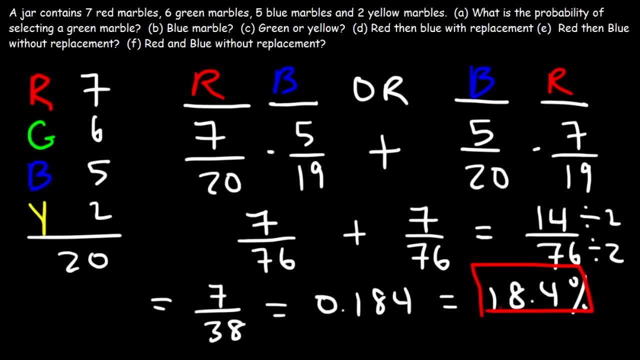 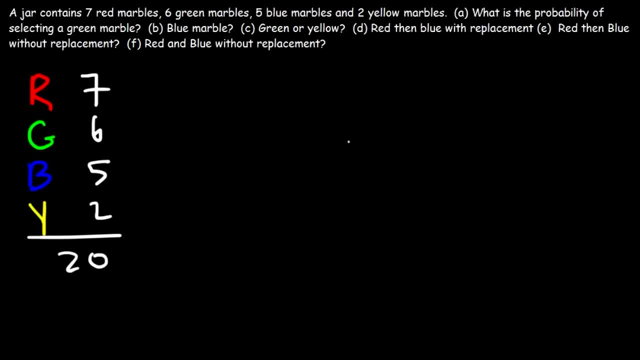 That's going to help you when solving probability problems. So anytime you see the word, or associate it with addition or sum, Whenever you see the word and associate it with multiplication. So just keep that in mind. So here's a question for you. 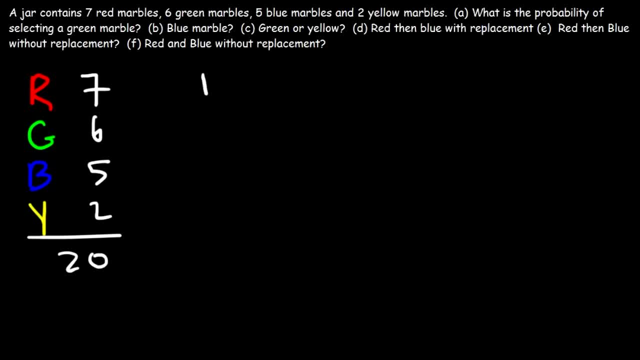 What is the probability of selecting a red marble, then a green marble? not, and So you want to get a red marble first and then a green marble on the second try, Or get in a blue marble and then a yellow marble on the second try. 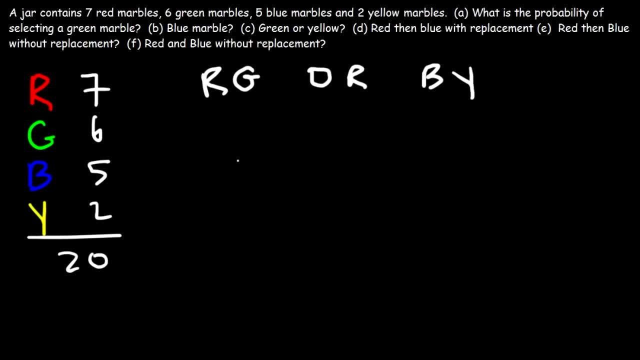 So go ahead and try to figure this out. So the probability of getting red and green, we need to multiply it. So it's going to be P of R. That's the probability of selecting a red marble And the probability of selecting a green marble. 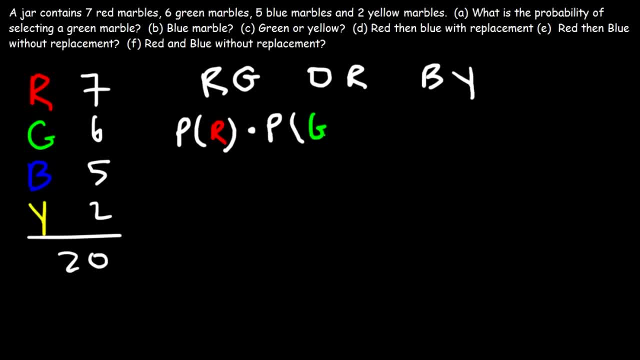 So we're going to multiply it by PG, And then we have an or statement, So that's going to be addition. The probability of getting a blue marble, that's PB, And the probability of getting a yellow marble, We'll call it a PY. 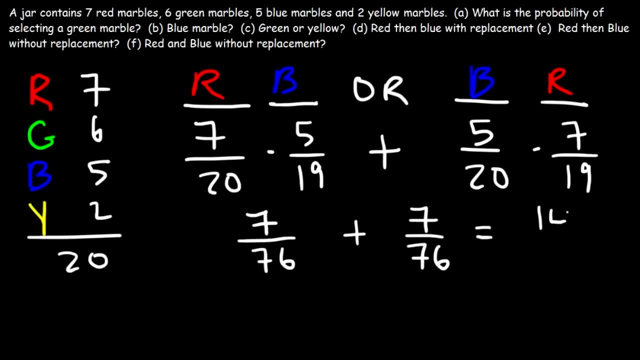 You have to double the answer, So it's 14 out of 76.. Now we can reduce this fraction. We can divide the top and the bottom by 2.. So this is going to turn into 7 over 38.. 7 over 38, that's 0.184.. 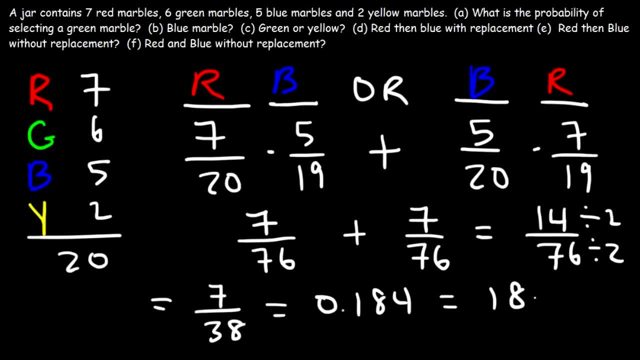 As a decimal, So there's an 18.4% chance of getting a red and a blue marble without replacement. The probability of not getting a red and a blue marble without replacement is 100 minus 18.4.. And that's 81.6% chance of not getting a red and blue. 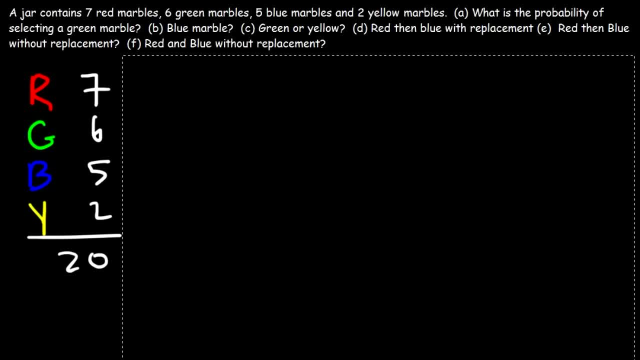 So now let's review A few important details That's going to help you when solving probability problems. So anytime you see the word, or associate it with addition or sum, Whenever you see the word and associate it with multiplication. So just keep that in mind. 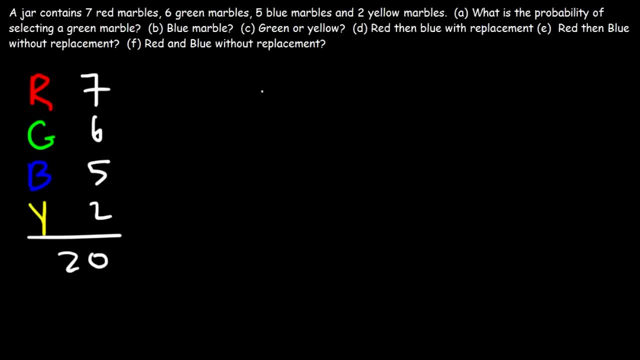 So here's a question for you: What is the probability of selecting a red marble, Then a green marble? Not. and So you want to get a red marble first and then a green marble on the second try, Or get in a blue marble and then a yellow marble on the second try. 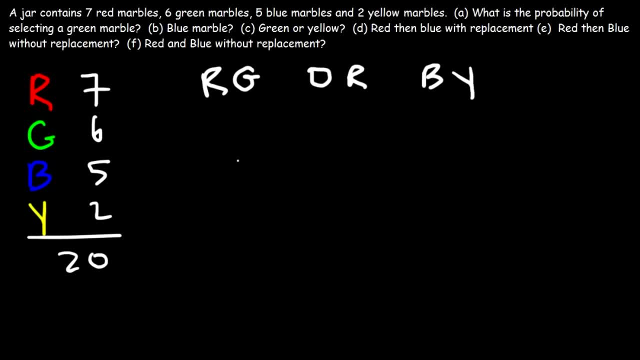 So go ahead and try to figure this out. So the probability of getting red and green, we need to multiply it. So it's going to be P Of R. That's the probability of selecting a red marble And the probability of selecting a green marble. 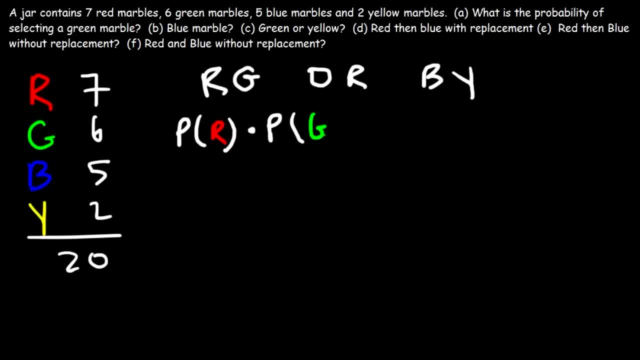 So we're going to multiply it by Pg And then we have an or statement, So that's going to be addition. The probability of getting a blue marble, that's Pb, And the probability of getting a yellow marble, we'll call it a Py.